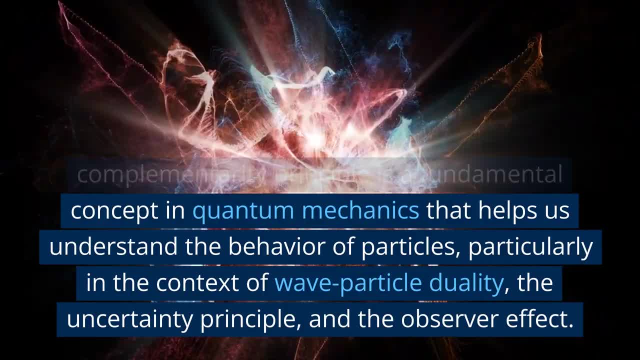 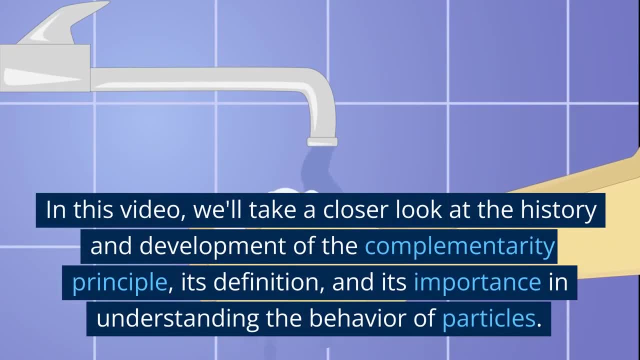 understand the behavior of particles, particularly in the context of wave-particle duality, the Uncertainty Principle and the Observer Effect. In this video, we'll take a closer look at the history and development of the Complementarity Principle, its definition and its importance in understanding the behavior of particles. 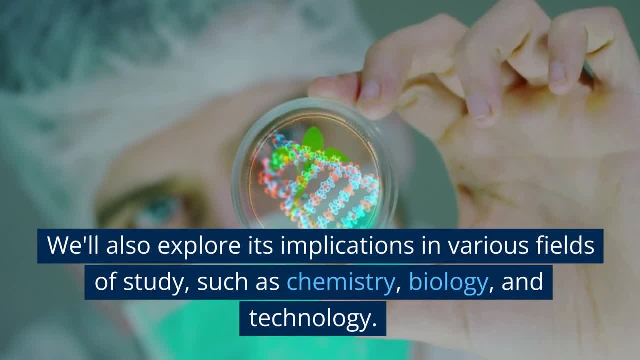 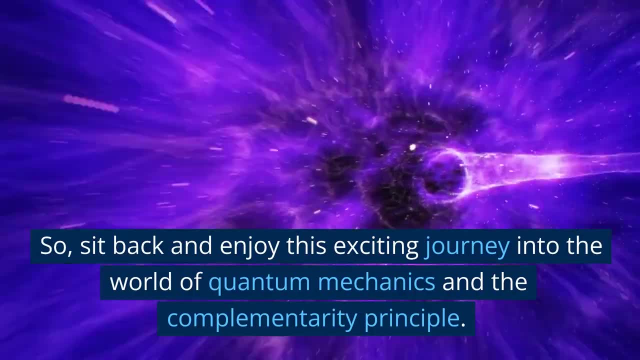 We'll also explore its implications in various fields of study, such as chemistry, biology and technology. So sit back and enjoy this exciting journey into the world of quantum mechanics and the Complementarity Principle. And, if you haven't already, be sure to subscribe. 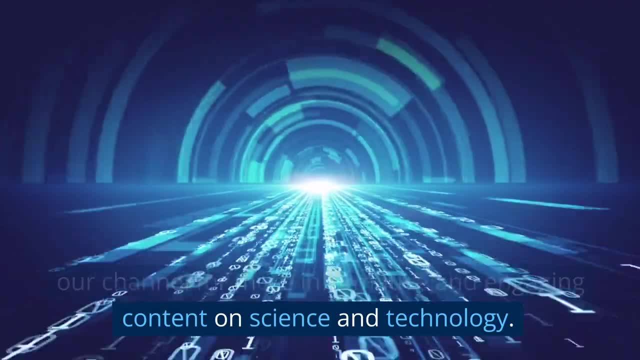 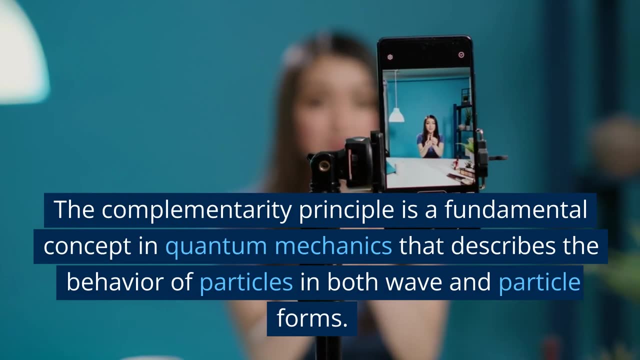 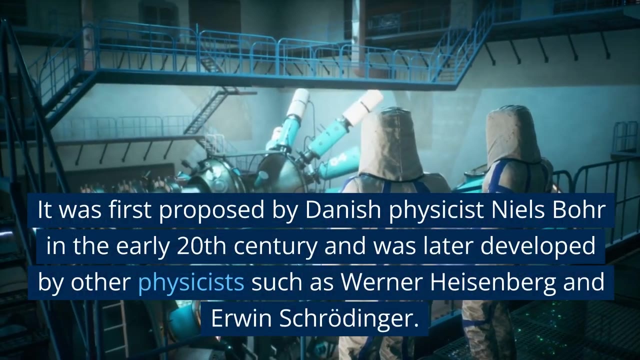 to our channel for more informative and engaging content on quantum mechanics. The Complementarity Principle is a fundamental concept in quantum mechanics that describes the behavior of particles in both wave and particle forms. It was first proposed by Danish physicist Niels Bohr in the early 20th century and was later developed by other physicists such as. 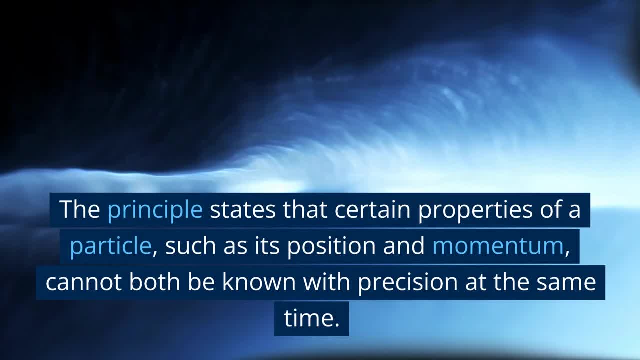 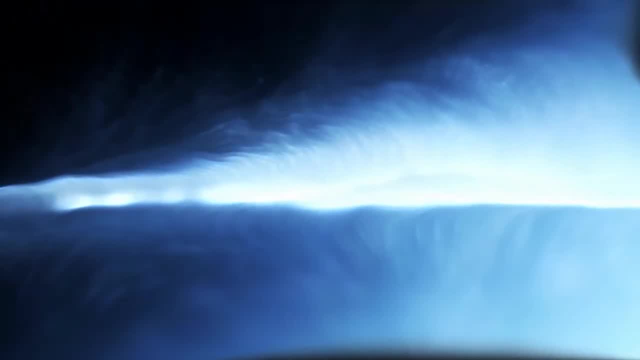 Werner Heisenberg and Erwin Schrödinger. The principle states that certain properties of a particle, such as its position and momentum, cannot both be known with precision at the same time. In other words, the more precisely one knows the position of a particle, the less precisely one can. 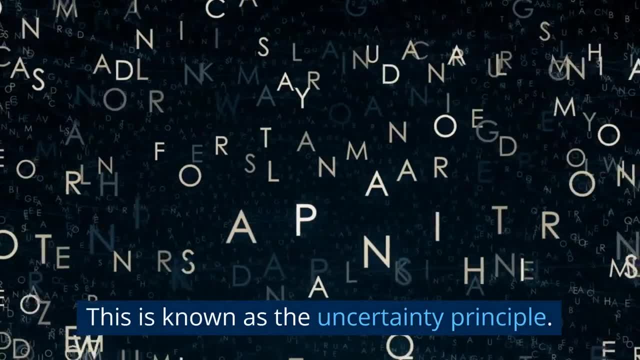 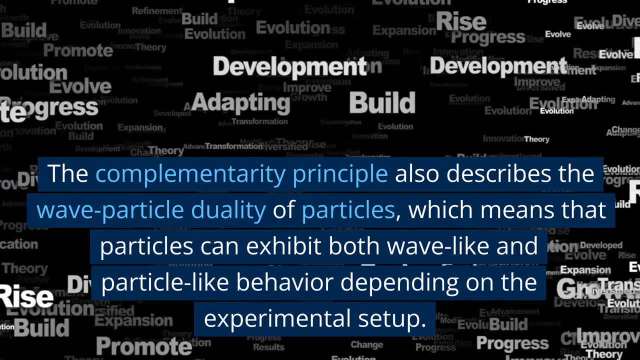 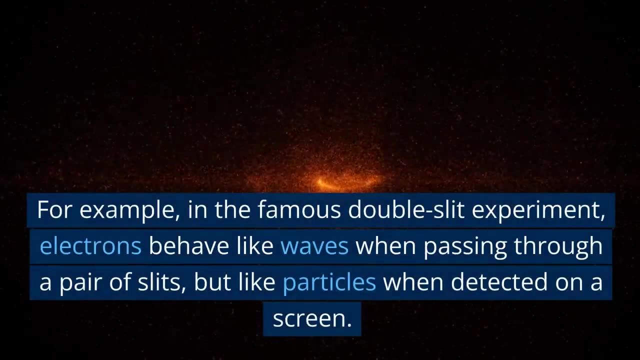 know its momentum and vice versa. This is known as the Uncertainty Principle. The Complementarity Principle also describes the wave-particle duality of particles, which means that particles can exhibit both wave-like and particle-like behavior depending on the experimental setup, For example in the famous double-split experiment. 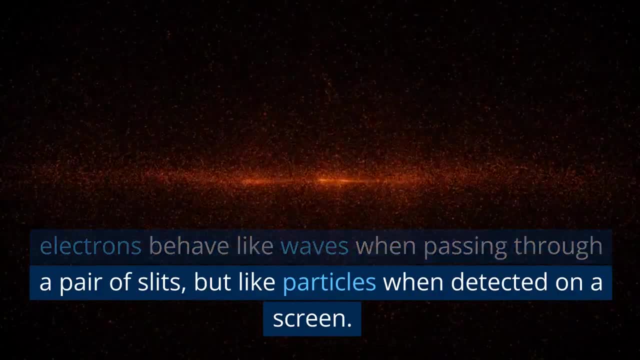 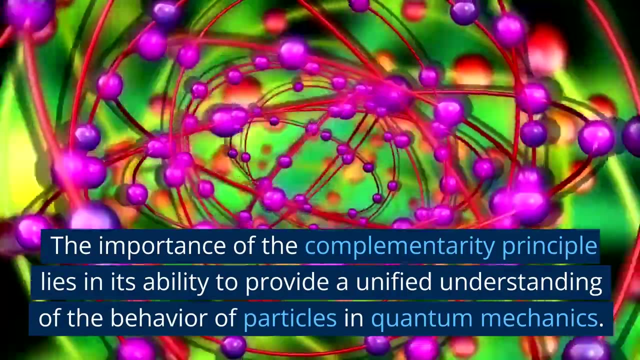 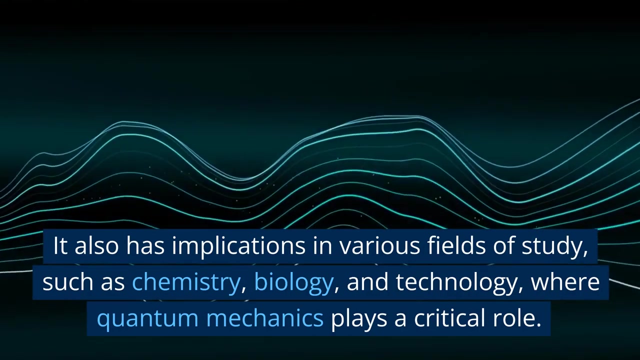 electrons behave like waves when passing through a pair of slips, but like particles when detected on a screen. The importance of the Complementarity Principle lies in its ability to provide a unified understanding of the behavior of particles in quantum mechanics. It also has implications in various fields of study such as chemistry, biology and technology. 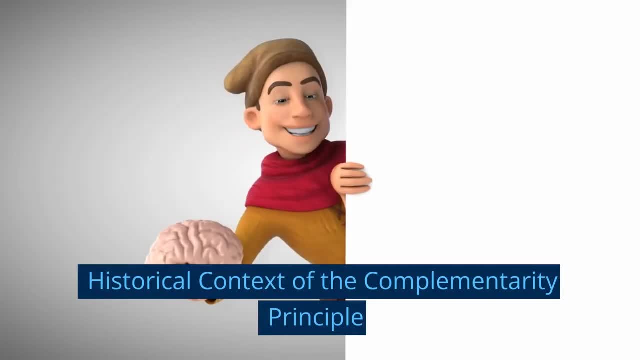 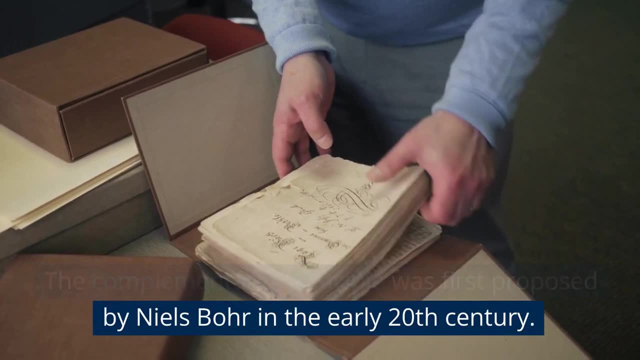 where quantum mechanics plays a critical role. Historical Context of the Complementarity Principle. The Complementarity Principle was first proposed by Niels Bohr in the early 20th century. Bohr was a Danish physicist who worked in the field of quantum mechanics for a long time. He was a 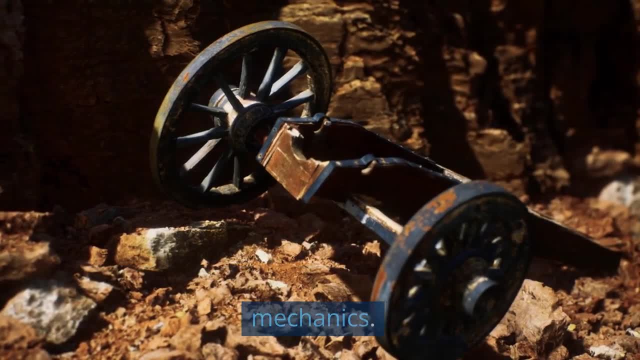 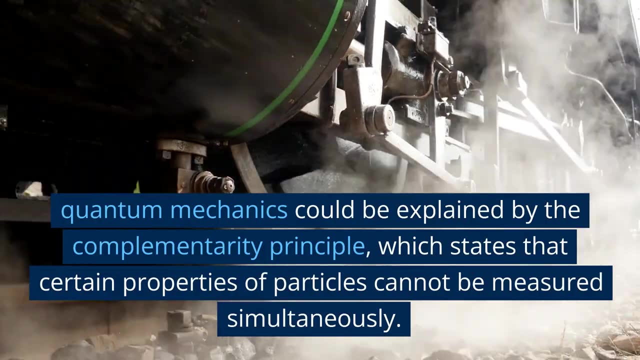 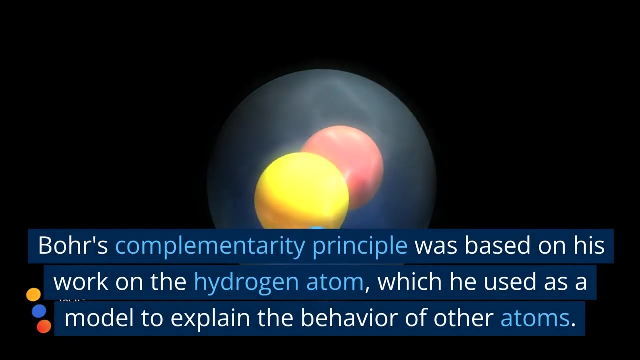 scientist who made significant contributions to the development of quantum mechanics. He proposed that the behavior of particles in quantum mechanics could be explained by the Complementarity Principle, which states that certain properties of particles cannot be measured simultaneously. Bohr's Complementarity Principle was based on his work on the hydrogen. 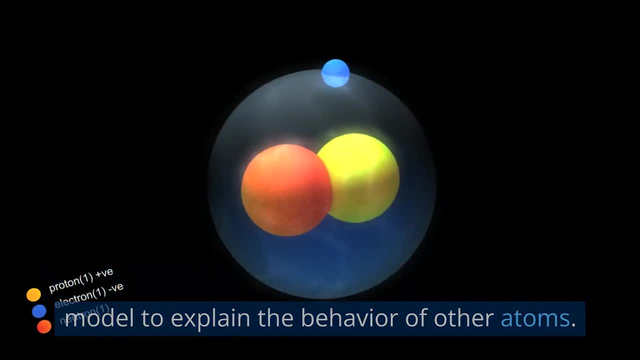 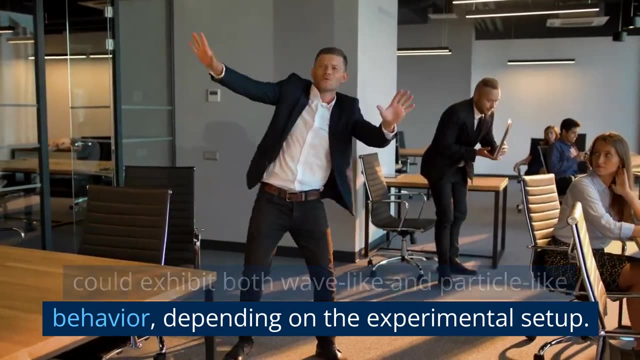 atom, which he used as a model to explain the behavior of other atoms. He argued that the electron in the hydrogen atom could exhibit both wave-like and particle-like behavior, depending on the experimental setup. Werner Heisenberg further developed the Complementarity Principle in 1927,. 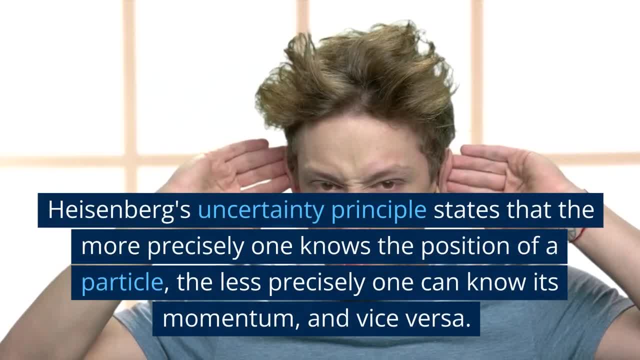 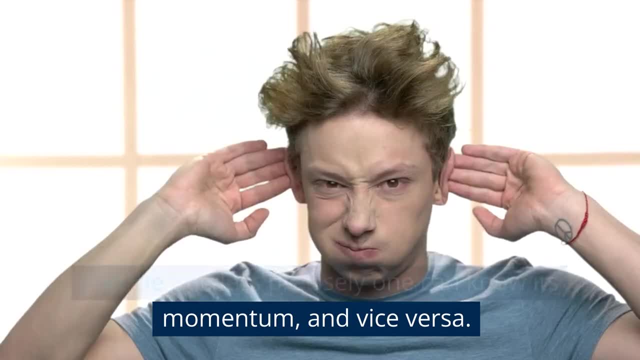 when he introduced the Uncertainty Principle. Heisenberg's Uncertainty Principle states that the more precisely one knows the position of a particle, the less precisely one can know its momentum, and vice versa. This principle was a direct consequence of the Complementarity. 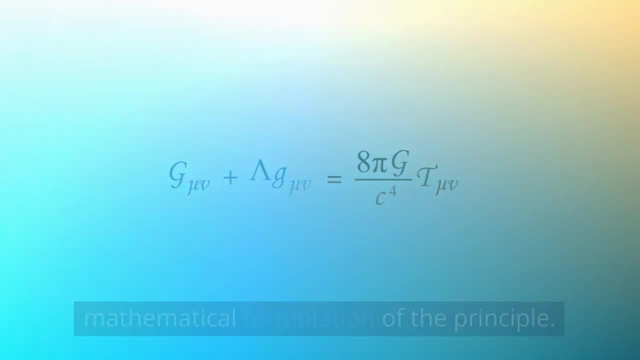 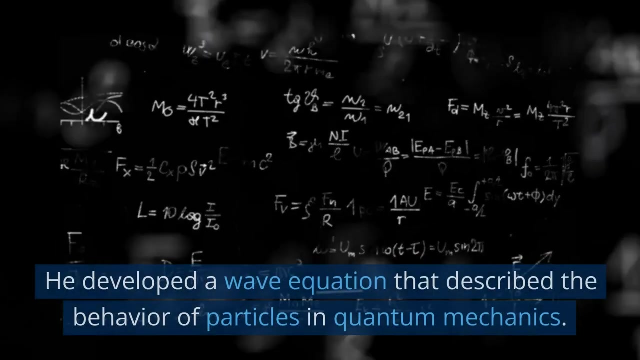 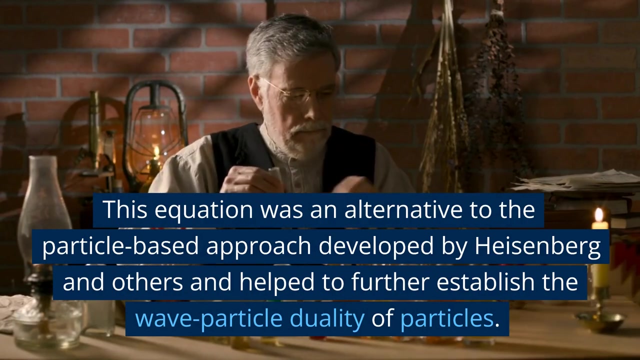 Principle and provided a mathematical formulation of the principle. Erwin Schrödinger also made significant contributions to the development of the Complementarity Principle. Erwin Schrödinger developed the Complementarity Principle for the use of particle-based quantum mechanics. He developed a wave equation that describes the behavior of particles in 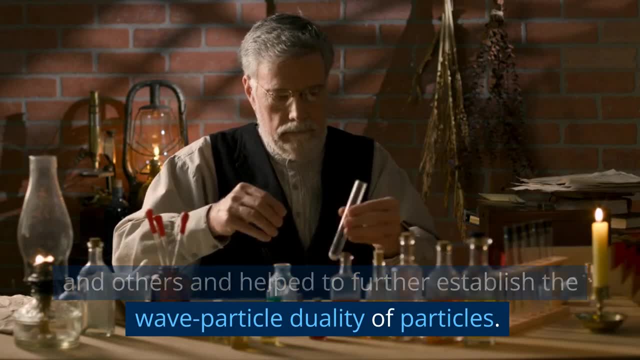 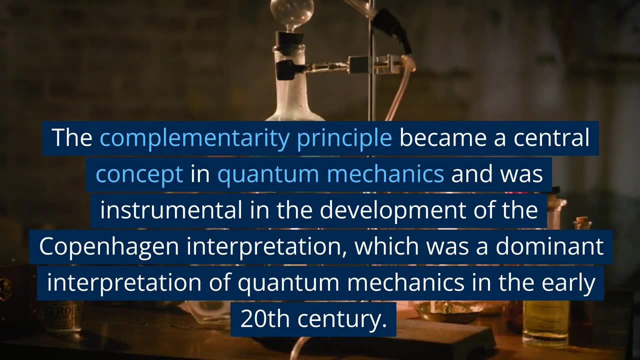 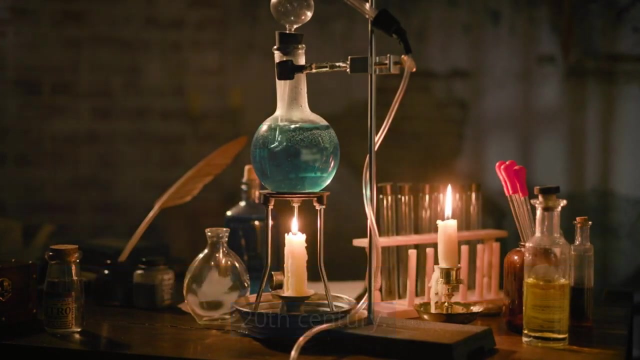 quantum mechanics. This equation was an alternative to the particle-based approach developed by Heisenberg and others and helped to further establish the wave-particle duality of particles. The Complementarity Principle became a central concept in quantum mechanics and was instrumental in the development of the Copenhagen Interpretation, which was a dominant interpretation of quantum. 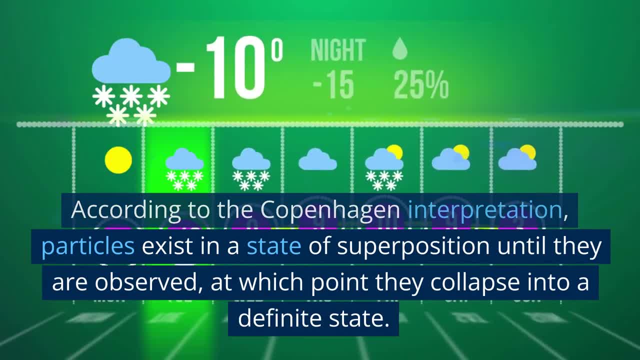 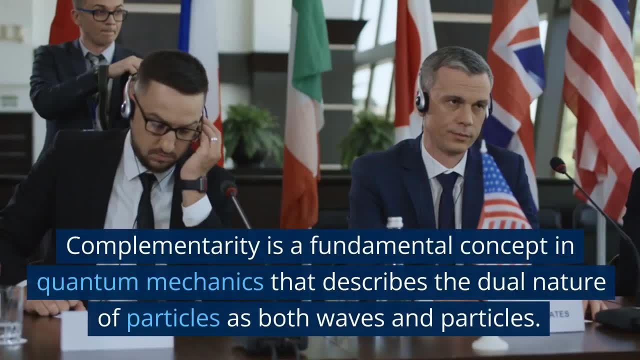 mechanics in the early 20th century exist in a state of superposition until they are observed, at which point they collapse into a definite state. The concept of complementarity- Complementarity- is a fundamental concept in quantum mechanics that describes the dual nature of particles as both waves and particles. 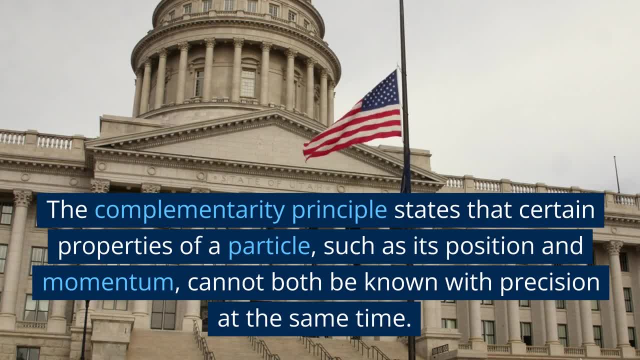 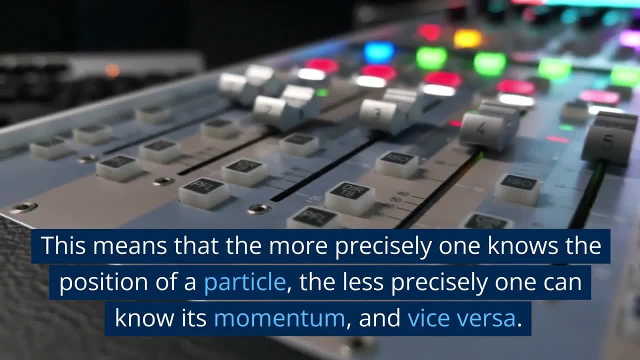 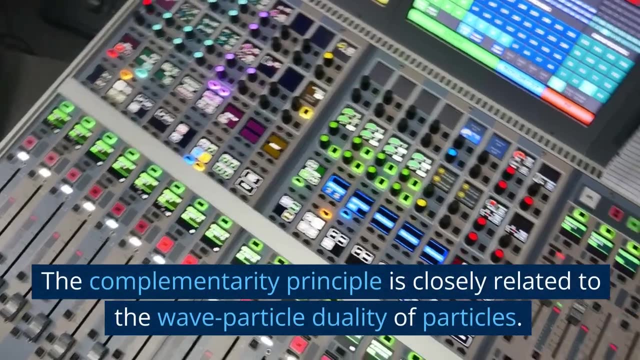 The complementarity principle states that certain properties of a particle, such as its position and momentum, cannot both be known with precision at the same time. This means that the more precisely one knows the position of a particle, the less precisely one can know its momentum, and vice versa. The complementarity principle 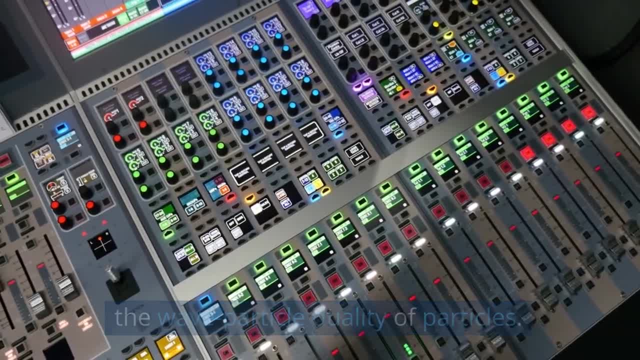 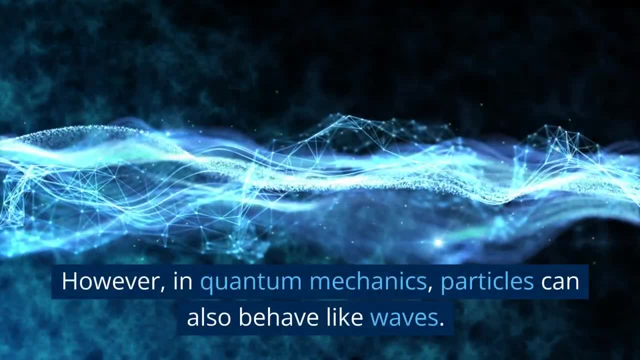 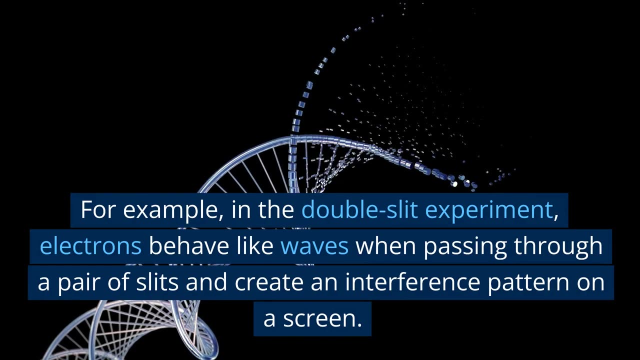 is closely related to the wave-particle duality of particles. In classical physics, particles are considered to be discrete entities that behave like particles. However, in quantum mechanics, particles can also behave like waves, For example in the double-slit experiment. 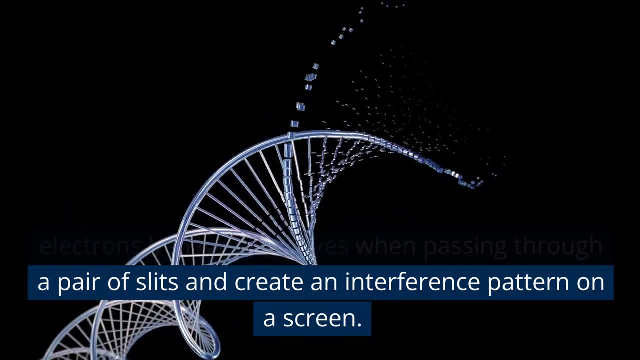 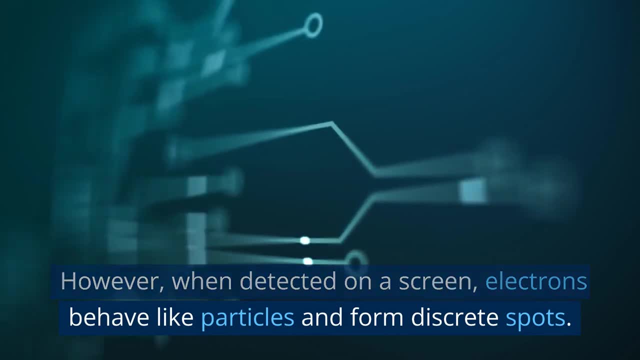 electrons behave like waves when passing through a pair of slits and create an interference pattern on the screen. However, in quantum mechanics, particles can also behave like waves. However, when detected on a screen, electrons behave like particles and form discrete spots. 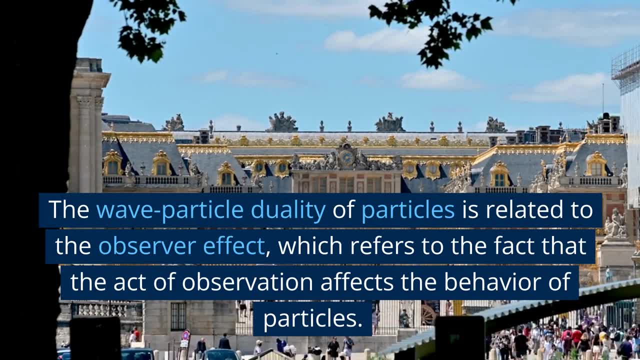 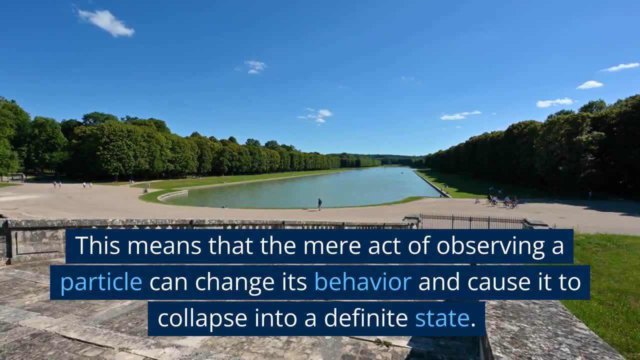 The wave-particle duality of particles is related to the observer effect, which refers to the fact that the act of observation affects the behavior of particles. This means that the mere act of observing a particle can change its behavior and cause it to collapse into a definite state. This is known as wave-function collapse. 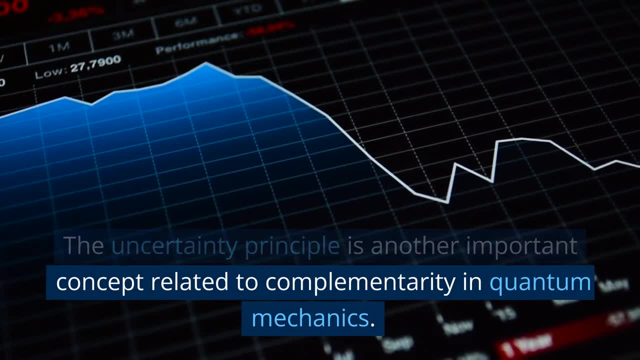 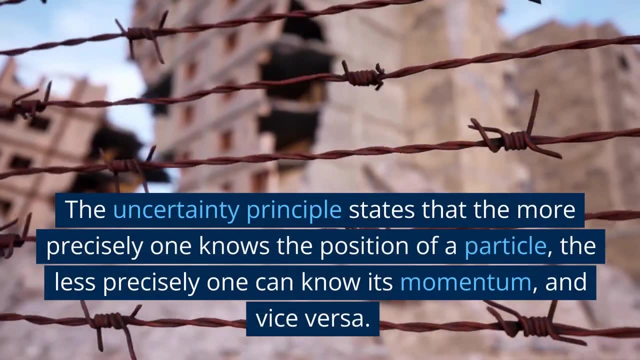 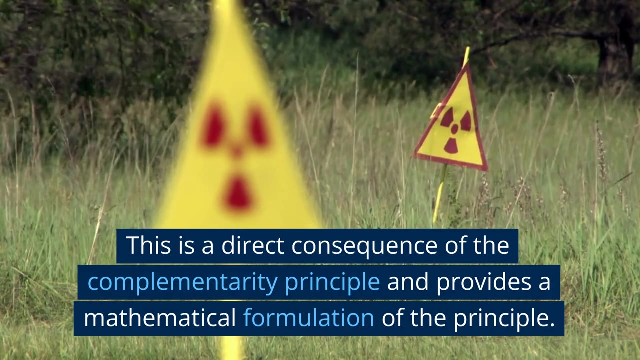 The uncertainty principle is another important concept related to complementarity. in quantum mechanics, The uncertainty principle states that the more precisely one knows the position of a particle, the less precisely one can know its momentum, and vice versa. This is a direct consequence of the complementarity principle and provides a mathematical formulation of the principle. 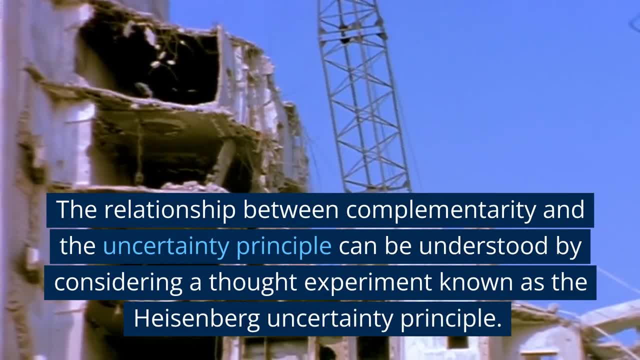 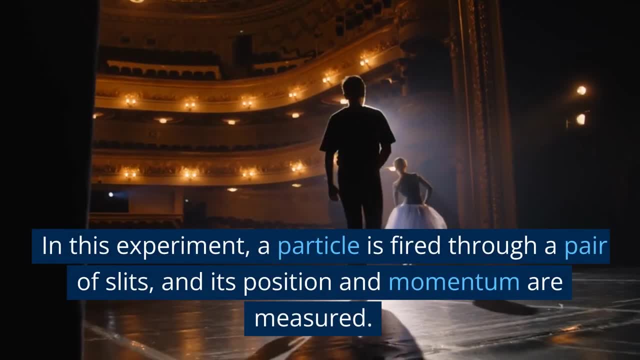 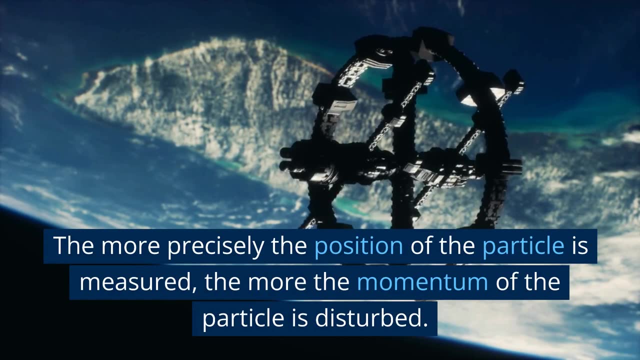 The relationship between complementarity and the uncertainty principle can be understood by considering a thought experiment known as the Heisenberg uncertainty principle. In this experiment, a particle is fired through a pair of slits and its position and momentum are measured. The more precisely the position of the particle is measured, the more the momentum of the particle 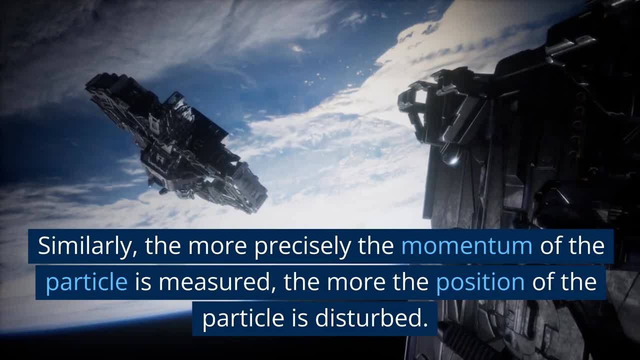 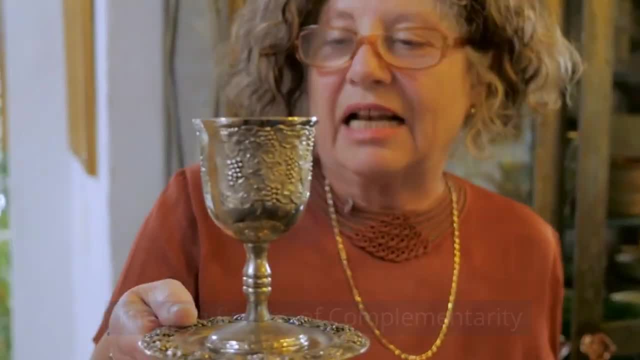 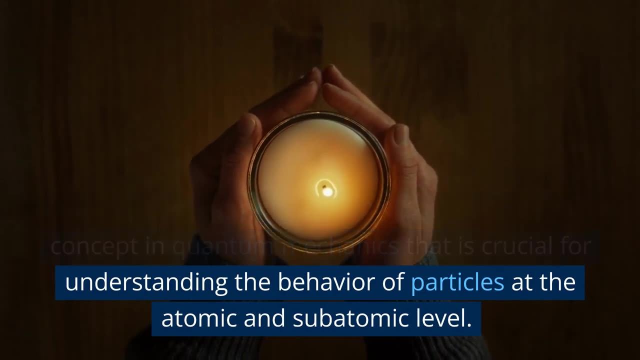 is disturbed. Similarly, the more precisely the momentum of the particle is measured, the more the position of the particle is disturbed. The Significance of Complementarity, The complementarity principle, is a fundamental concept in quantum mechanics that is crucial for understanding the behavior of particles at the atomic and subatomic level. 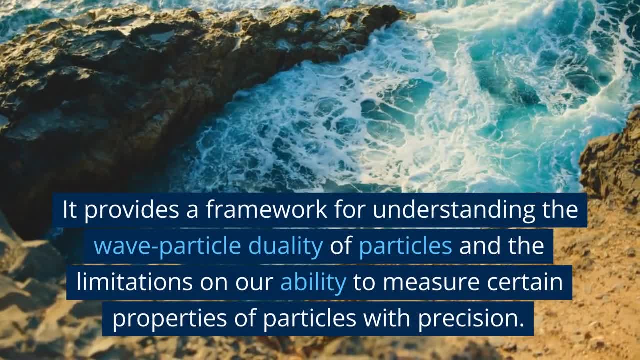 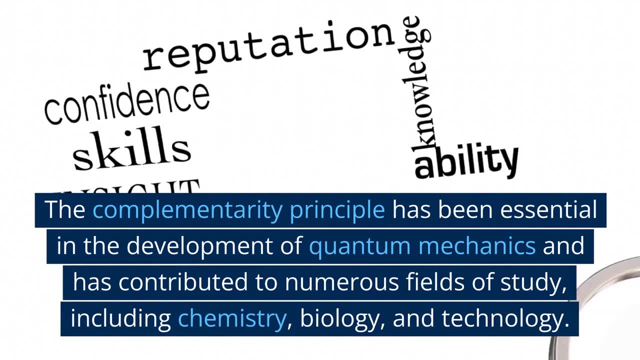 It provides a framework for understanding the wave-particle duality of particles and the limitations on our ability to understand them. The result is our ability to measure certain properties of particles with precision. the complementarity principle has been essential in the development of quantum mechanics and has 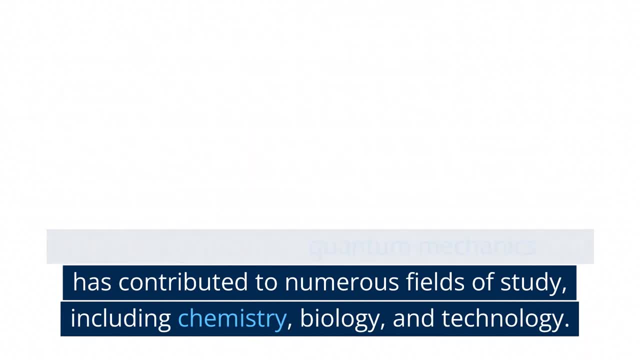 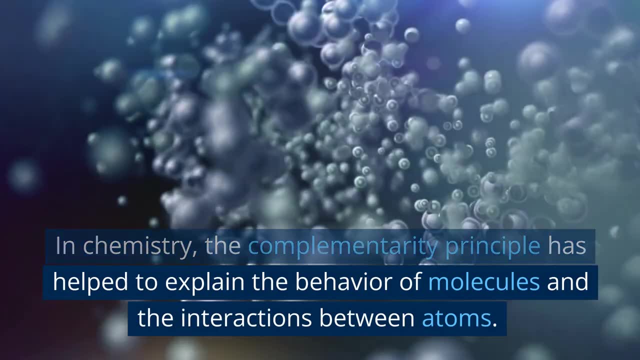 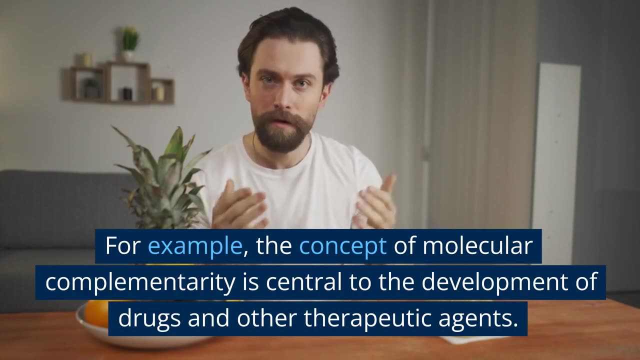 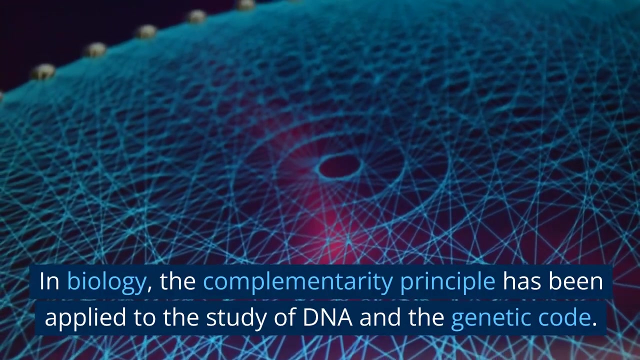 contributed to numerous fields of study, including chemistry, biology and technology. in chemistry, the complementarity principle has helped to explain the behavior of molecules and interactions between atoms. for example, the concept of molecular complementarity is central to the development of drugs and other therapeutic agents. in biology, the complementarity principle has been applied to the study of DNA and the genetic code. 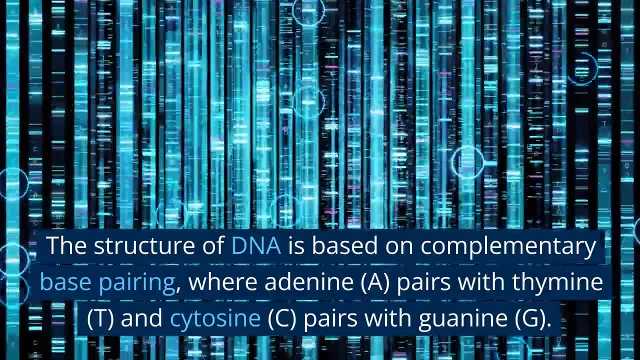 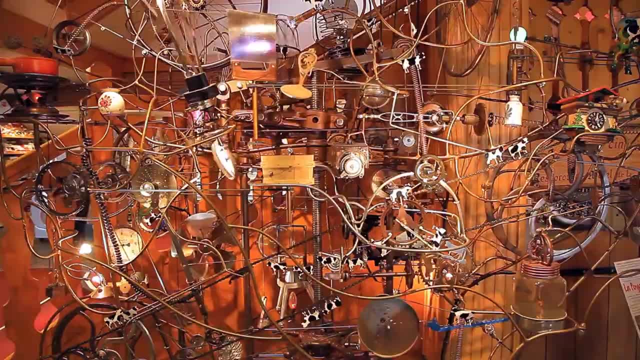 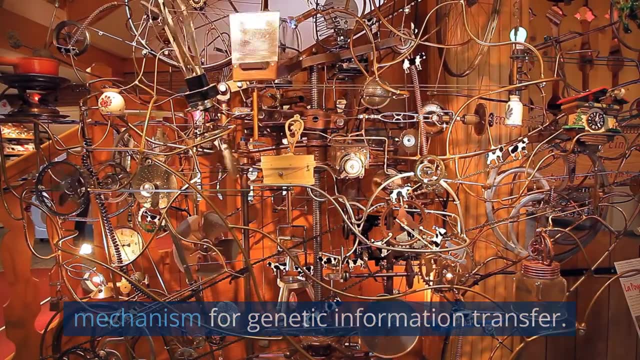 The structure of DNA is based on complementary base pairing, where adenine A pairs with thymine T and cytosine C pairs with guanine G. This pairing is essential for the replication and transcription of DNA and provides a fundamental mechanism for genetic information transfer. 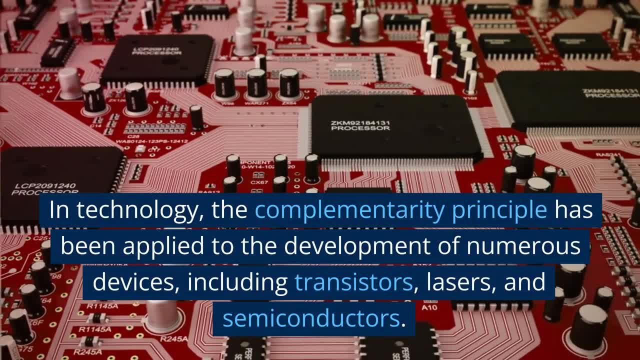 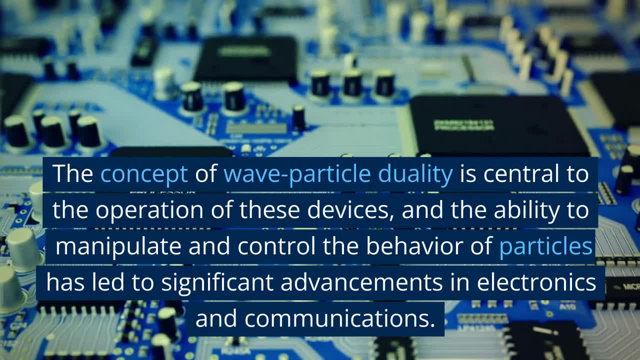 In technology, the complementarity principle has been applied to the development of numerous devices, including transistors, lasers and semiconductors. The concept of wave-particle duality is central to the operation of these devices and the ability to manipulate and 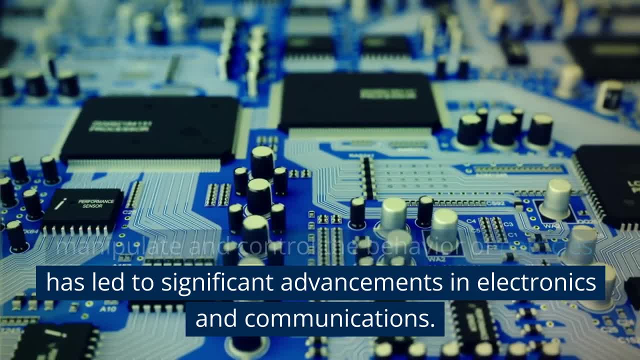 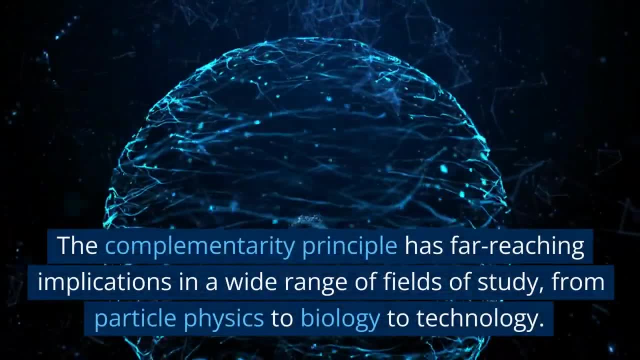 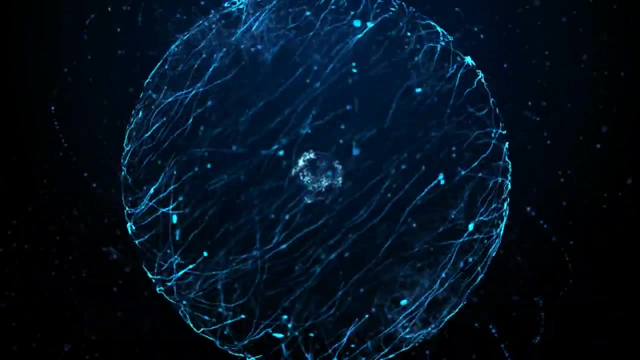 control the behavior of particles has led to significant advancements in electronics and communications. Implications of complementarity in different fields. The complementarity principle has far-reaching implications in a wide range of fields of study, from particle physics to biology to technology. In this section, 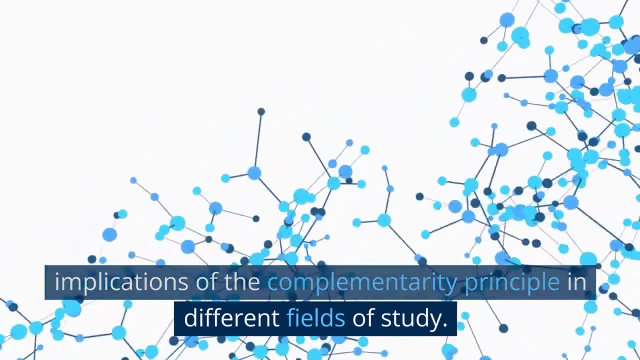 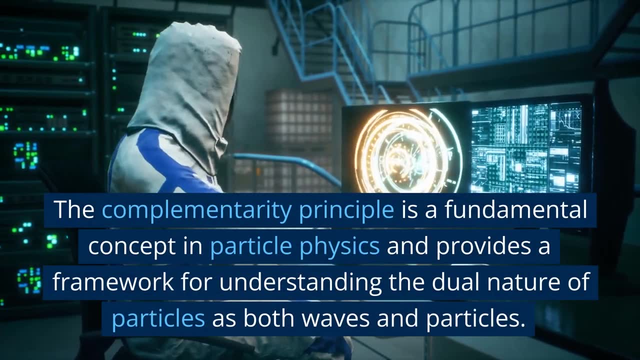 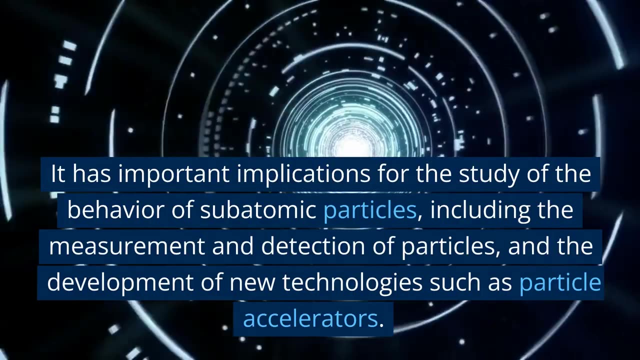 we will explore some of the implications of the complementarity principle in different fields of study. Particle physics: The complementarity principle is a fundamental concept in particle physics and provides a framework for understanding the dual nature of particles as both waves and particles. It has important implications for the study of the behavior of subatomic particles. 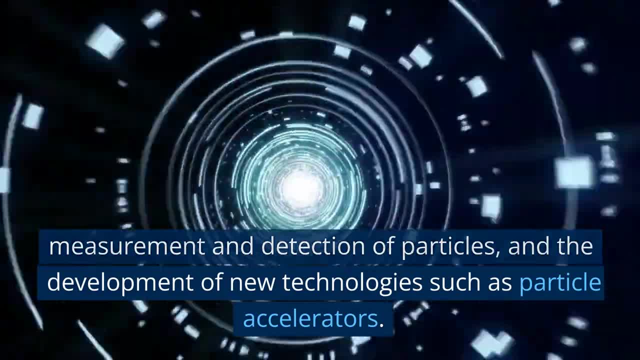 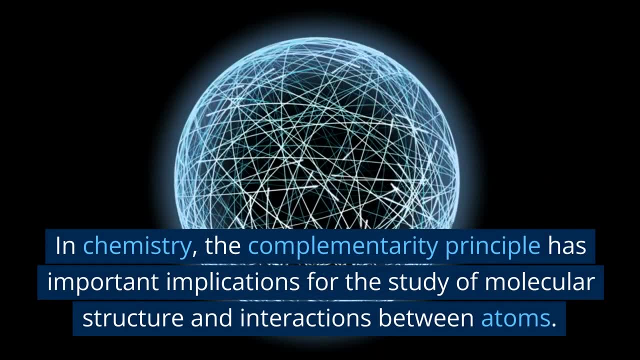 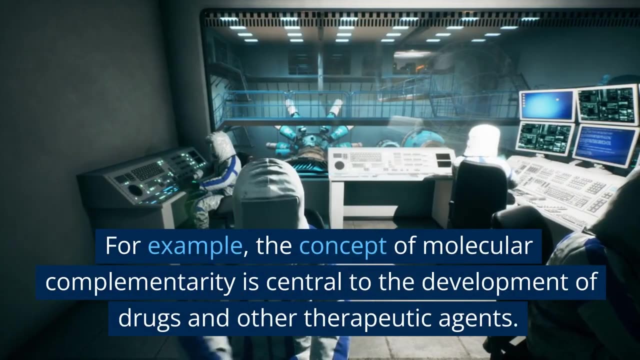 including the measurement and detection of particles and the development of new technologies such as particle accelerators. Chemistry: In chemistry, the complementarity principle has important implications. for the study of molecular structure and interactions between atoms, For example, the concept of molecular complementarity is central. 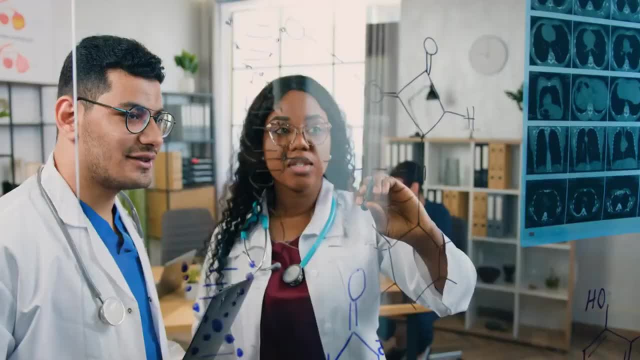 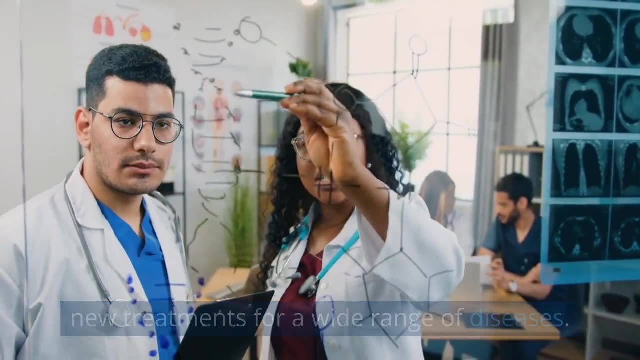 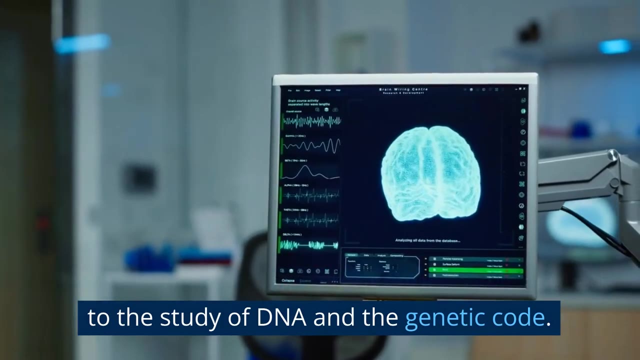 to the development of drugs and other therapeutic agents. Understanding the complementary nature of molecular interactions is essential for developing new treatments for a wide range of diseases. Biology: In biology, the complementarity principle is applied to the study of DNA and the genetic functions ofeez. The structure of DNA is based on complementary base pairing, which is essential for 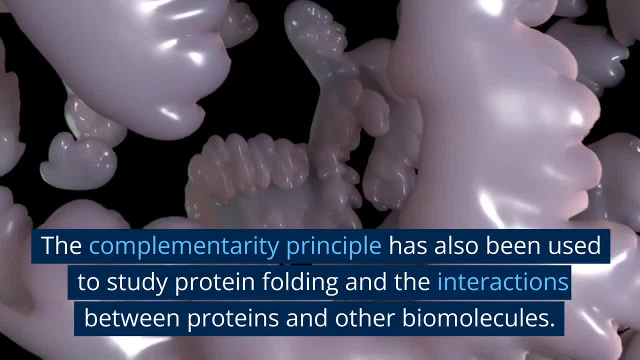 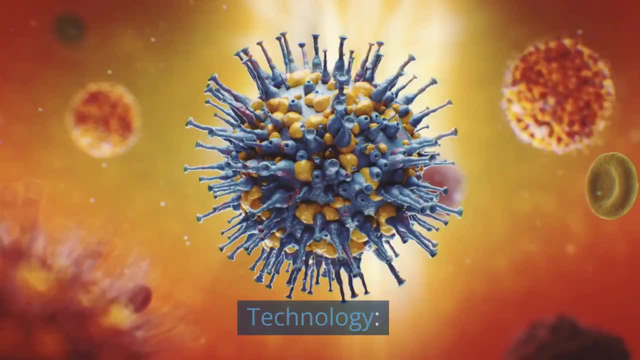 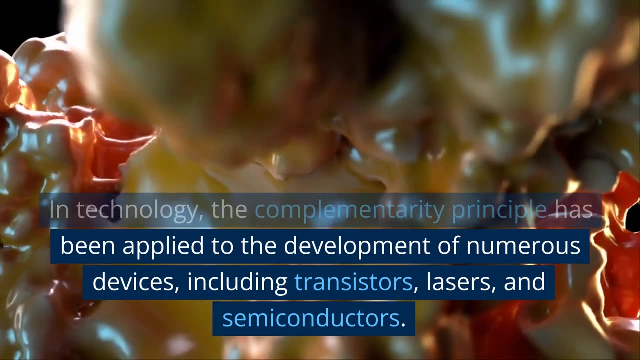 the replication and transcription of genetic information. The complementarity principle has also been used to study protein folding and the interactions between proteins and other biomolecules. Technology In technology, the complementarity principle has been applied to the development of numerous devices, including transistors, lasers and semiconductors. The concept of wave-particle duality is central to the operation of theserow. 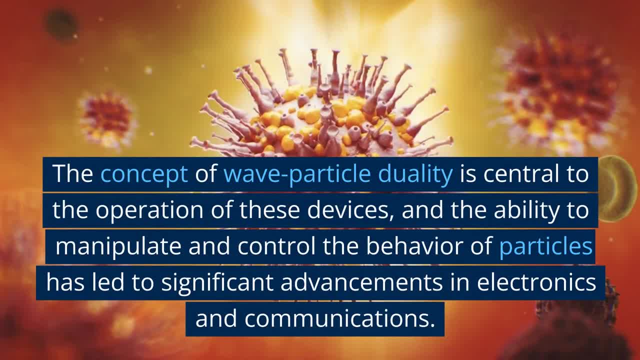 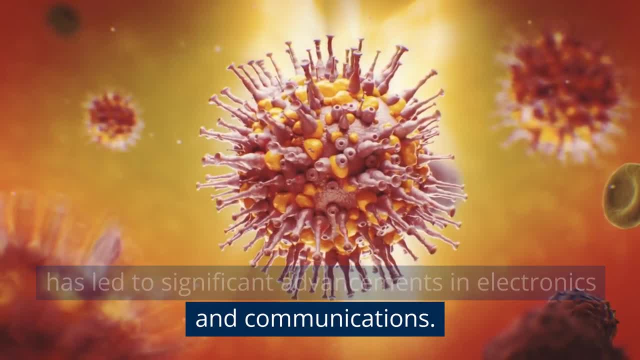 The concept of wave-particle duality is central to the operation of these mediums. For example, this could Ñl devices, and the ability to manipulate and control the behavior of particles has led to significant advancements in electronics and communications. nature of reality and human knowledge. the 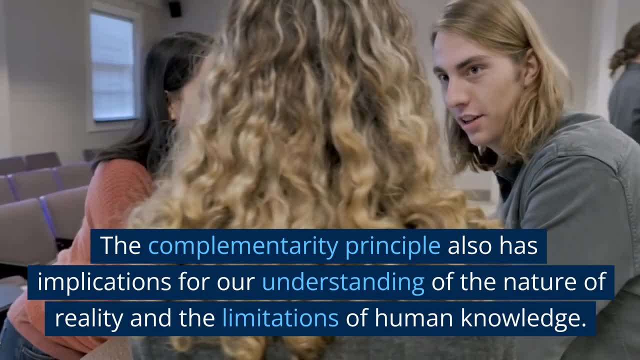 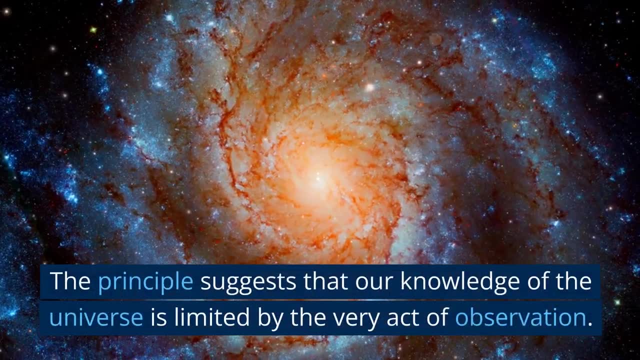 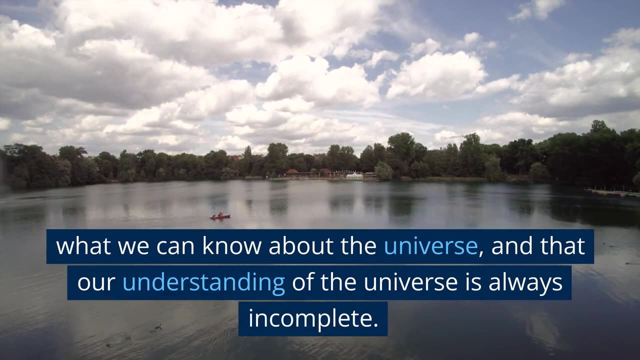 complementarity principle also has implications for our understanding of the nature of reality and the limitations of human knowledge. the principle suggests that our knowledge of the universe is limited by the very act of observation. it suggests that there are fundamental limits to what we can know about the universe and that our understanding of the universe is always incomplete. 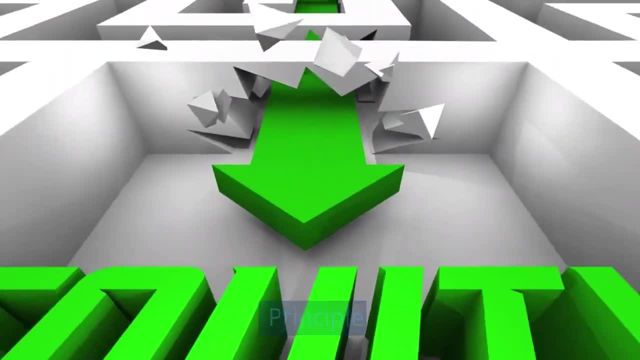 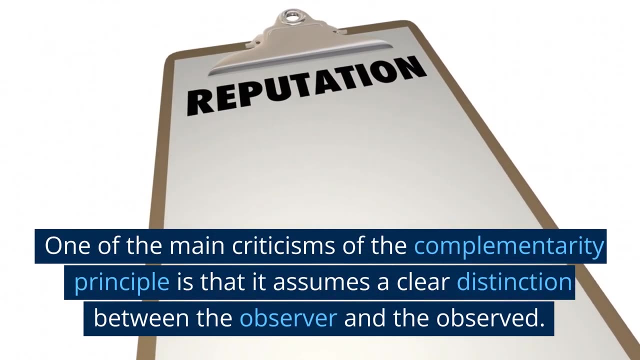 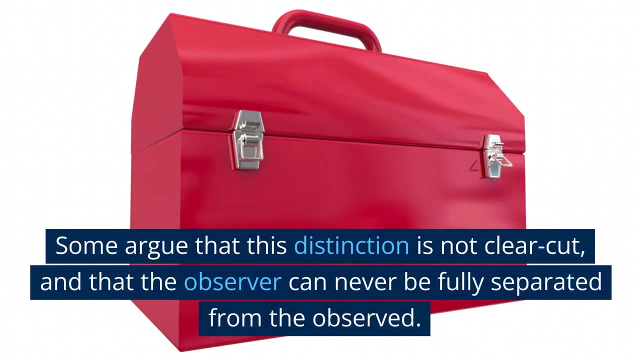 criticisms and challenges to the complementarity principle. the complementarity principle has been a subject of debate and criticism since its inception. one of the main criticisms of the complementarity principle is that it assumes a clear distinction between the observer and the observed. some argue that this distinction is not clear-cut. 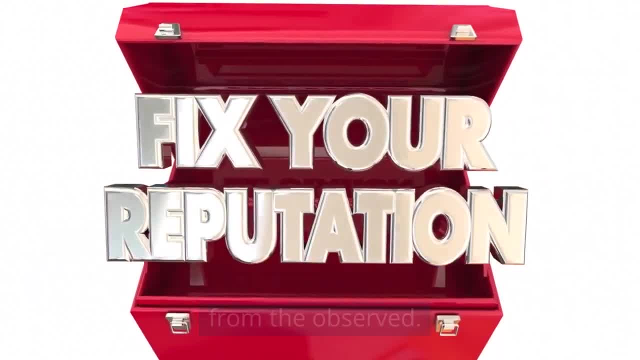 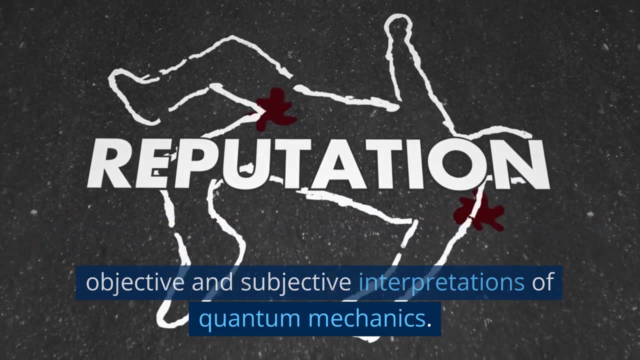 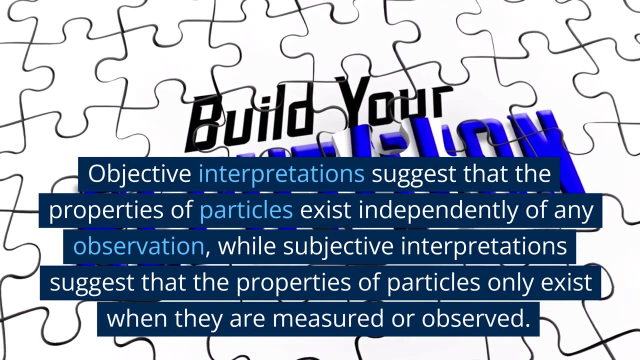 and that the observer can never be fully separated from the observed. another challenge to the complementarity principle arises from the ongoing debate between objective and subjective interpretations of quantum mechanics. objective interpretations suggest that the properties of particles exist independently of any observation, while subjective interpretations suggest that the 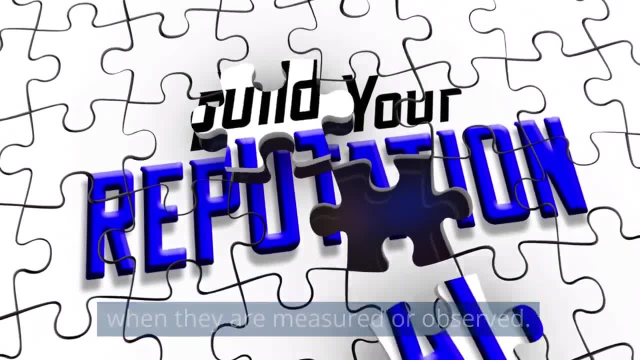 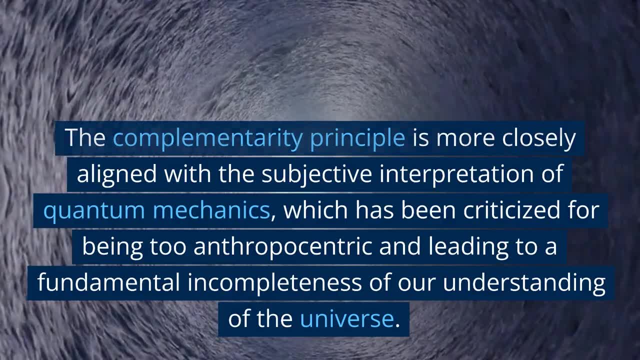 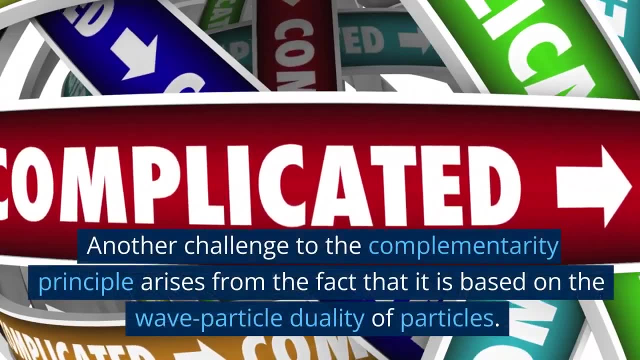 properties of particles only exist when they are measured or observed. the complementarity principle is more closely aligned with the subjective interpretation of quantum mechanics, which has been criticized for being too anthropocentric and leading to a fundamental incompleteness of our understanding of the universe. another challenge to the complementarity principle: 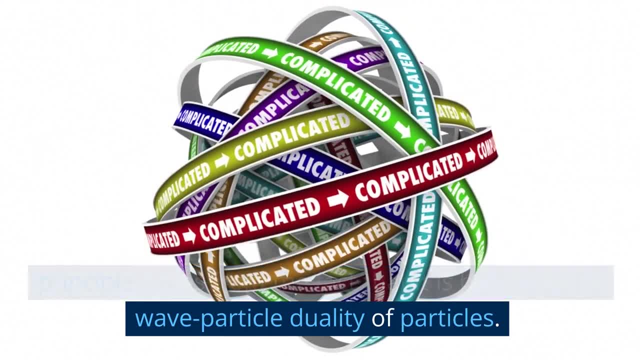 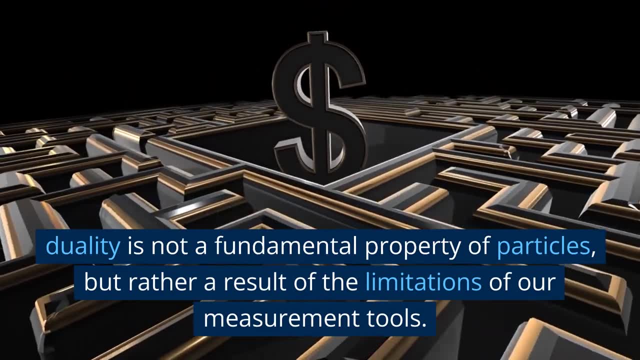 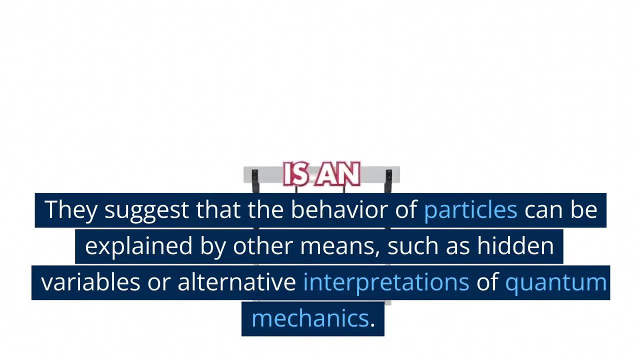 arises from the fact that it is based on the wave particle duality of particles. some researchers argue that the wave particle duality is not a fundamental property of particles, but rather a result of the limitations of our measurement tools. they suggest that the behavior of particles can be explained by other means, such as hidden variables. 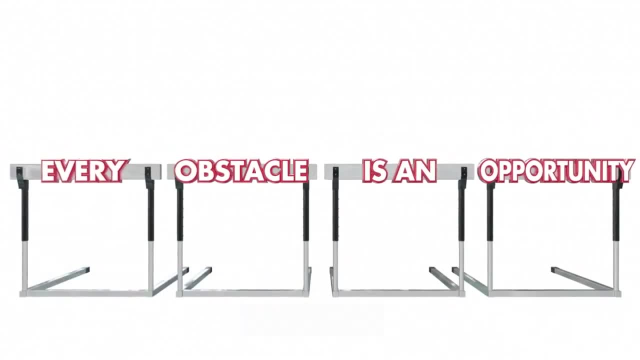 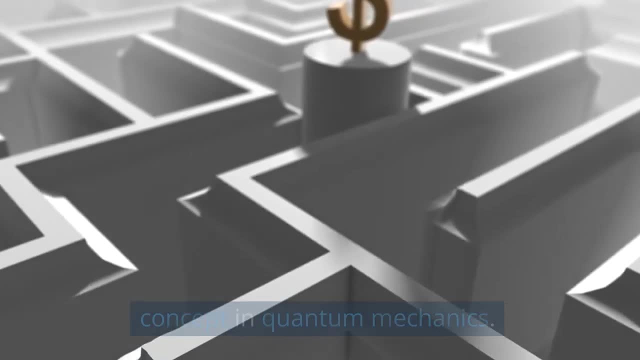 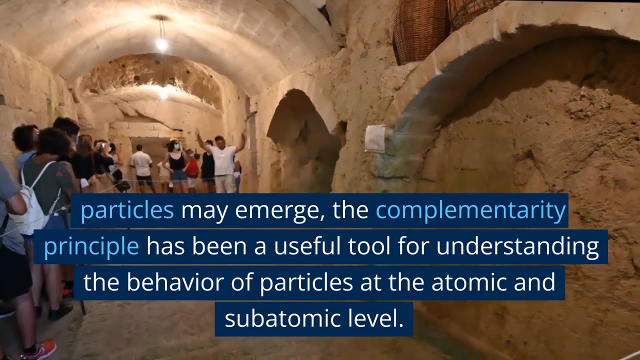 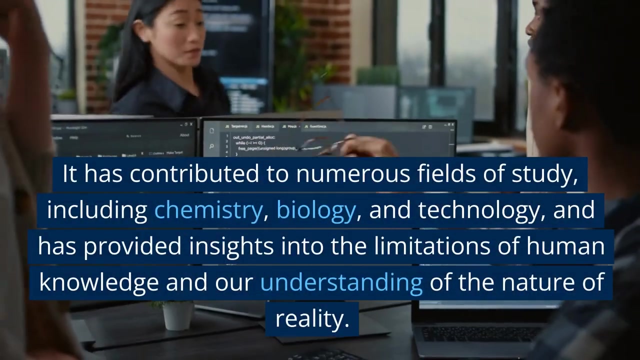 or alternative interpretations of quantum mechanics. despite these criticisms and challenges, the complementarity principle remains a fundamental concept in quantum mechanics. while alternative explanations for the behavior of particles may emerge, the complementarity principle has been a useful tool for understanding the behavior of particles at the atomic and subatomic level. it has contributed to numerous fields of study. 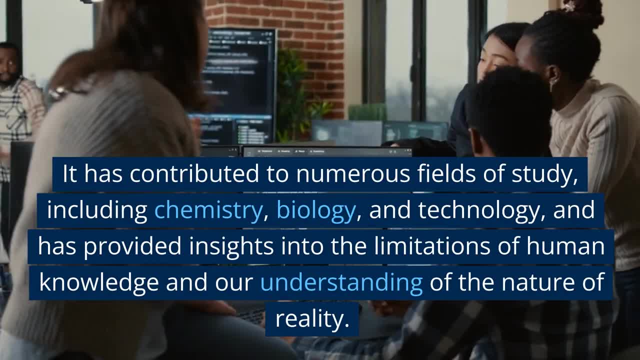 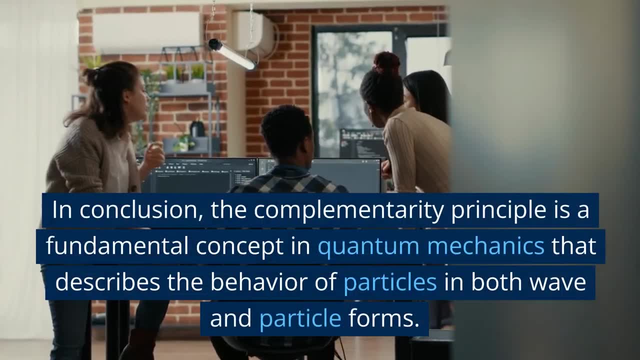 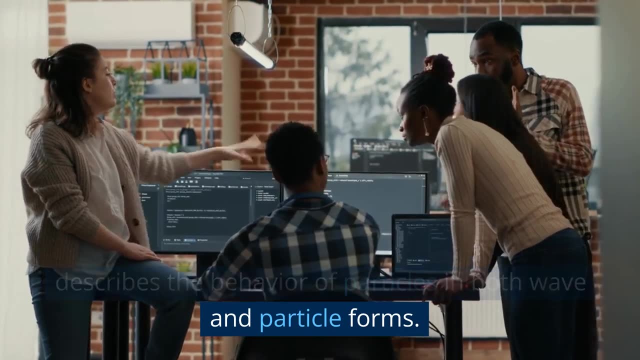 including chemistry, biology and technology, and has provided insights into the limitations of human knowledge and our understanding of the nature of reality. in conclusion, the principle is a fundamental concept in quantum mechanics that describes the behavior of particles in both wave and particle forms, Its historical development and significance. 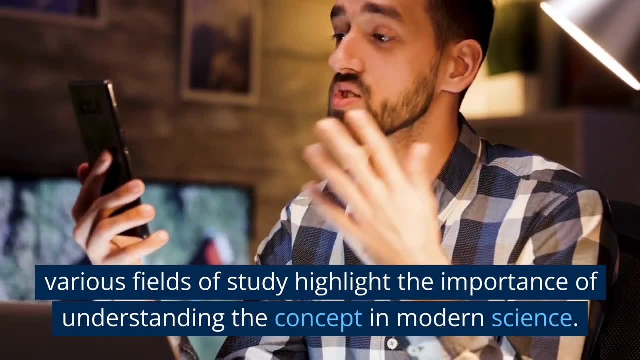 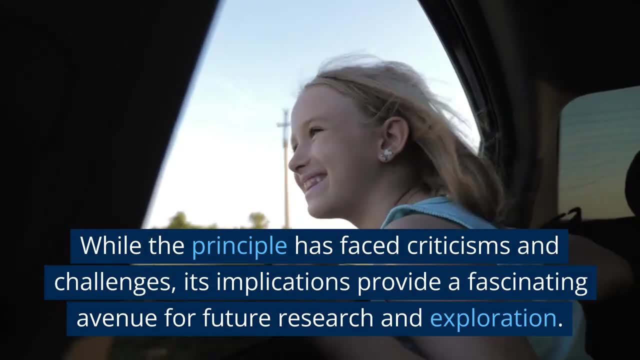 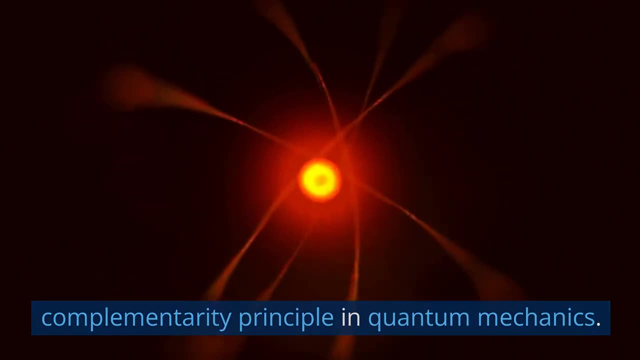 in various fields of study highlight the importance of understanding the concept in modern science. While the principle has faced criticisms and challenges, its implications provide a fascinating avenue for future research and exploration. Thank you for watching this video on the complementarity principle in quantum mechanics. We hope that this video has provided